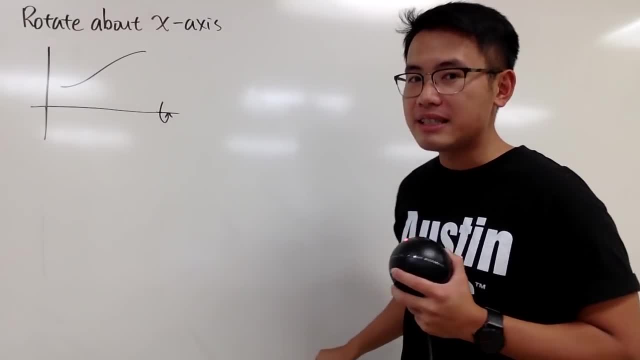 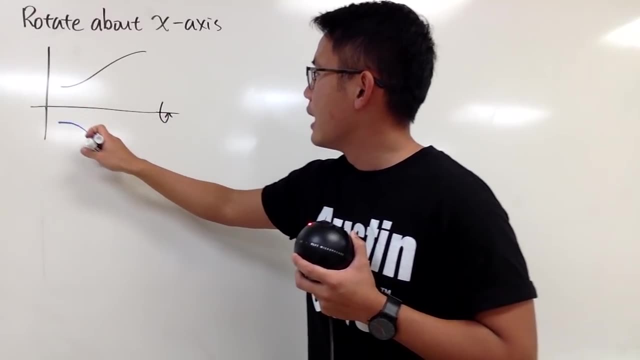 this portion of the curve and I will take that and rotate about the x-axis. So we go this way and we can do what we did in the volume video. I can first draw a mirror image like this and then at the end we can just put down this to make it three-dimensional looking. However, 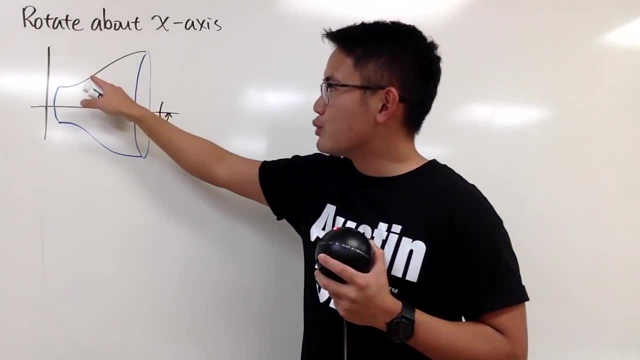 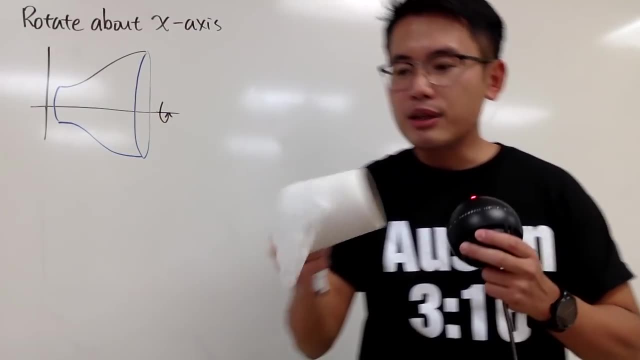 though, unlike the volume video, I am not going to draw a perfect disc. I'm not going to draw a small horizontal line and then rotate. That's not enough, because we actually don't have that situation. Just take a look of the roll of the toilet paper. If you draw a little horizontal, 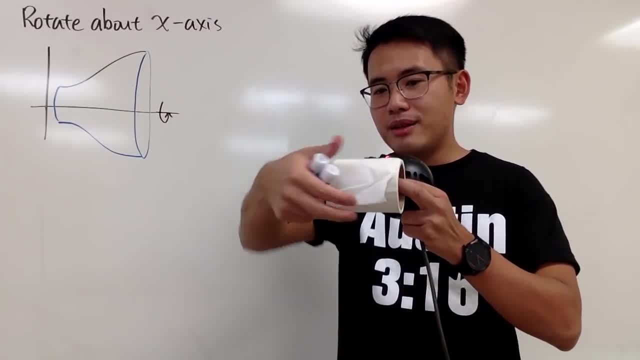 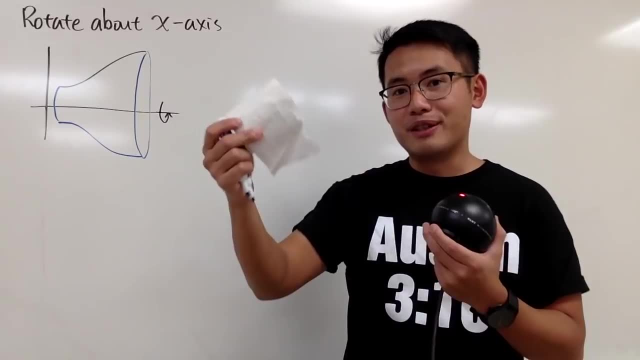 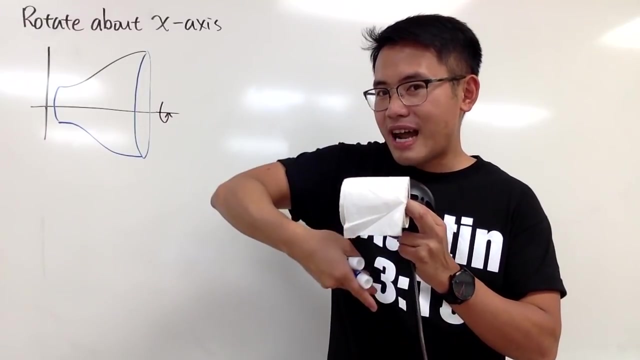 line. then you're talking about roll of toilet paper. You rotate that. then you're talking about this lateral area, The lateral area of this cylinder right. However, you can see that this is being curved up, So it's like this, and you have to rotate that. You actually have to talk about the lateral area of a. 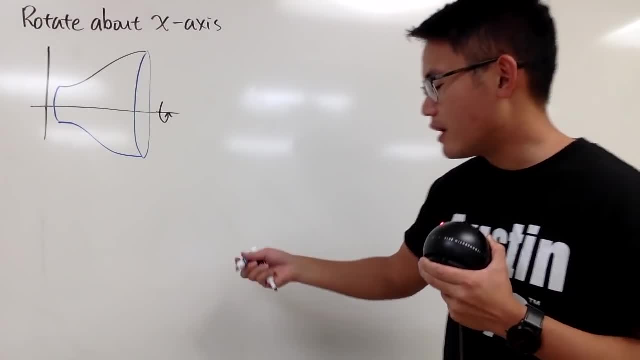 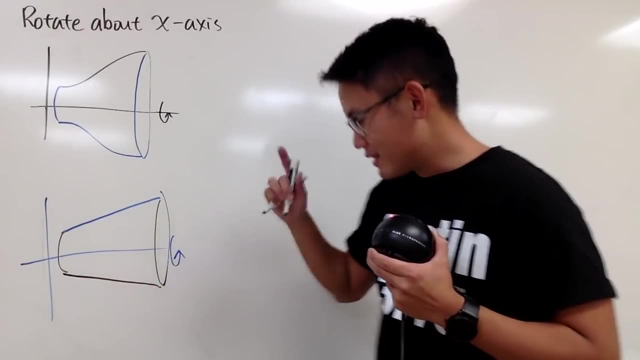 cone. Well, just part of it. And to make this super clear, let's just consider the following. Now, what kind of picture do you see? It's pretty much a part of the cone, right? So that's what I meant earlier. So, right here, what you have to do is you have to draw a little horizontal line. 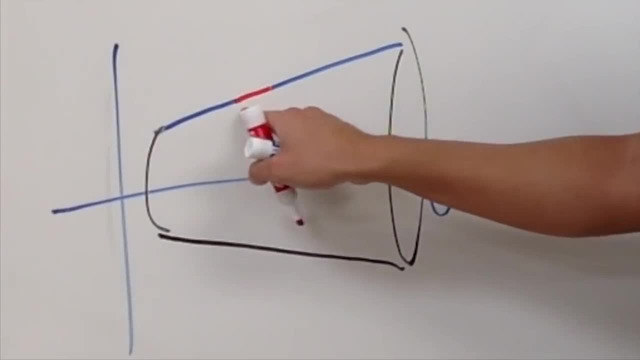 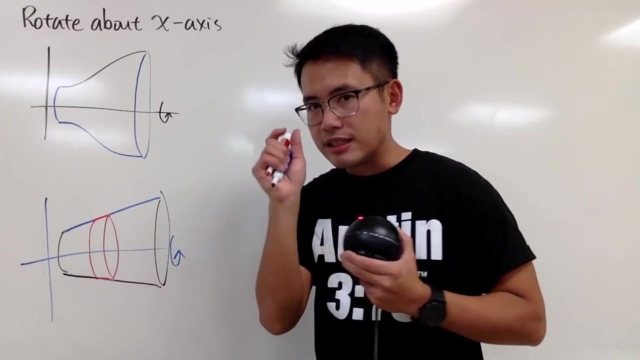 and what you have to do is, because it's a cone, you can just take a small portion, like stand right here and rotate like this. And now here's a label, and I'm going to do that later on with this real quick, But let's focus on this. This right here is just a small change in the arc length. 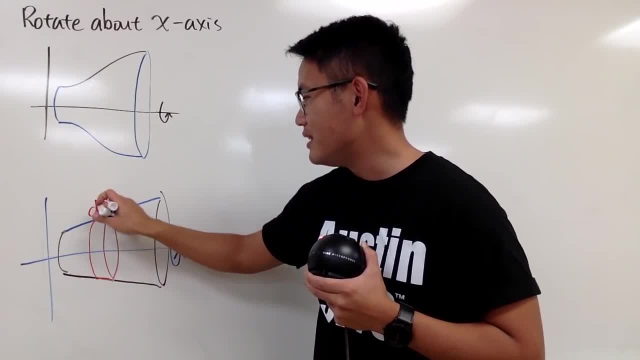 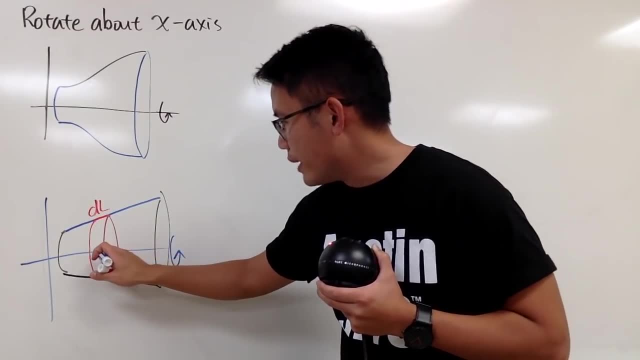 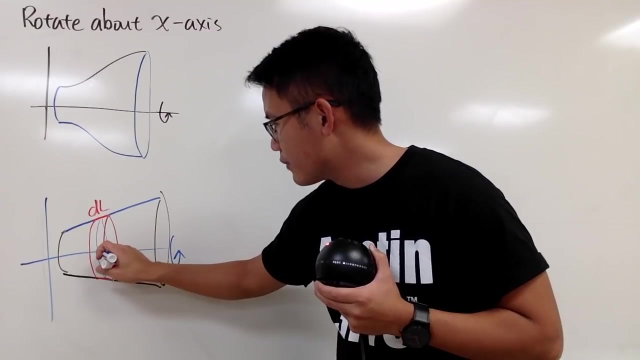 technically, even though this is a straight line, But I will still call this to be DL And you need to draw the radius of the middle right here, the middle portion. I will just put this down from here to here, And of course this is just the vertical distance, so we'll call that to be Y. 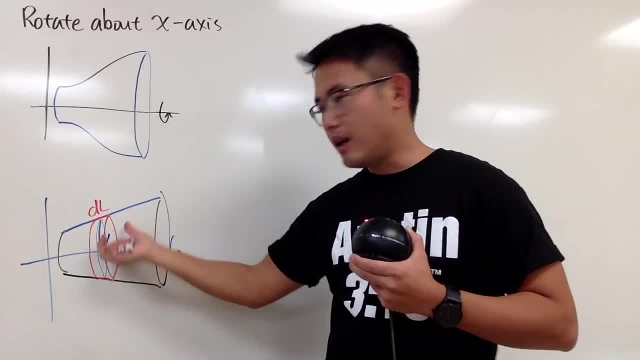 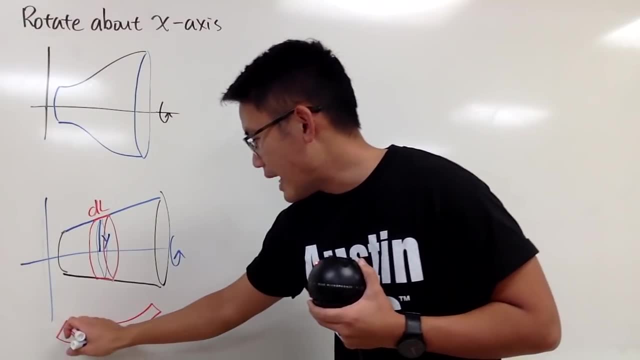 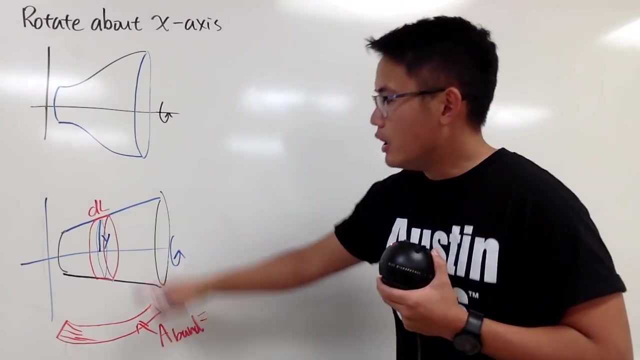 If you have this bend, you know, just cut it from the cone and then open it. you are going to end up with. the picture looks like this And the area of this bend is the following: The area of the bend- once again, refer back to my previous video. you need to know this, which is Y, And what you do is: 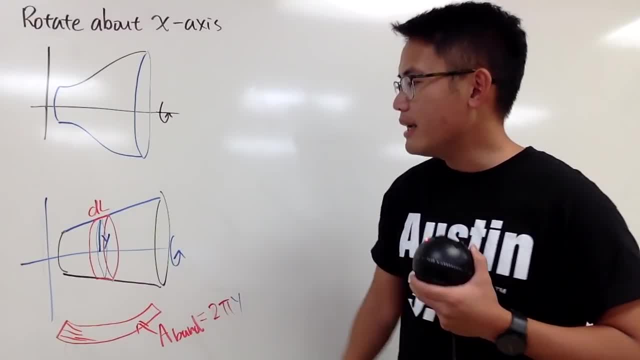 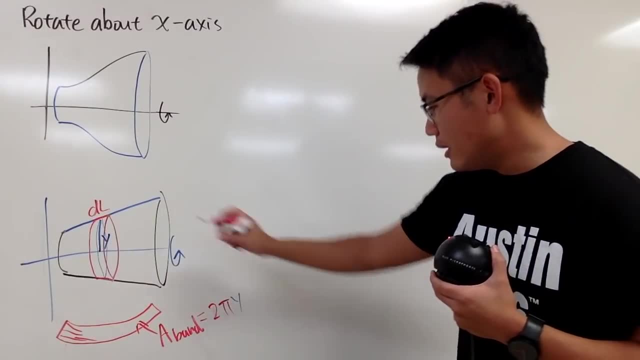 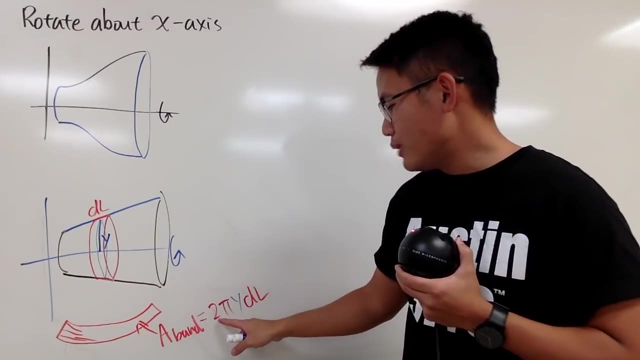 two pi times the radius Y, and this is the middle radius. okay, Two pi times Y and then times this length which, based on our labeling, is DL, like that. Well, yes, notice that we do have the two pi Y and that is the circumference. If you go from this as your radius, 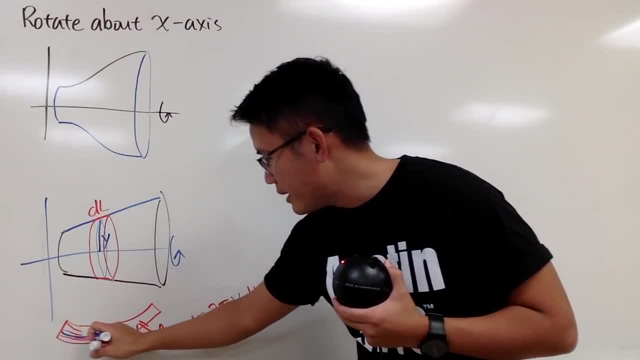 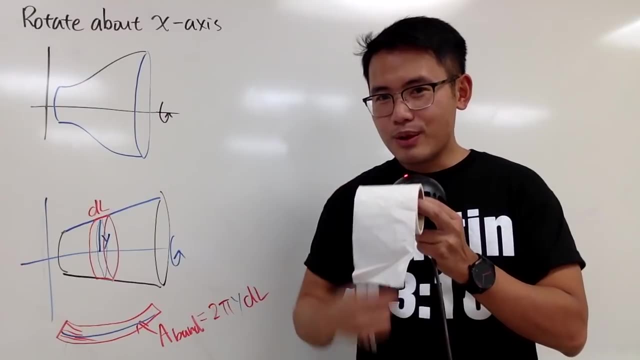 round it, meaning if you just look at that, you open it just like this: The middle radius is R, I mean it's Y, And then go around it one time you have the two pi Y. So that's how you can. 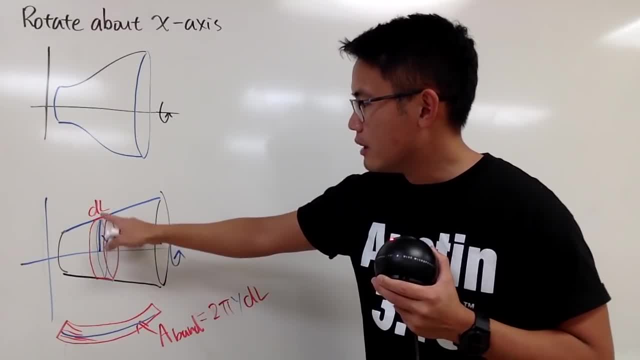 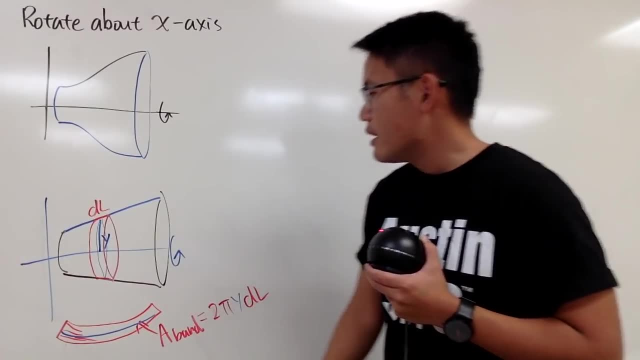 remember it, It's pretty much a circumference based on this circle, and then you multiply by the length of the side, which is the DL. That's pretty much all Well. for the curve situation, same thing, And you need a middle, which is 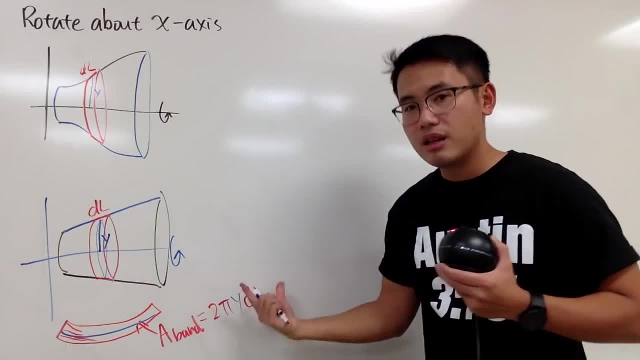 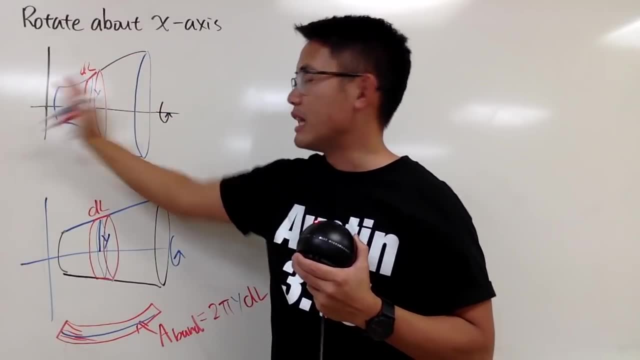 Y, you need that which is DL, which is, once again, you need the area of the band. As usual, you need to find this area of the band and then you add them up, that's all. So here we go. 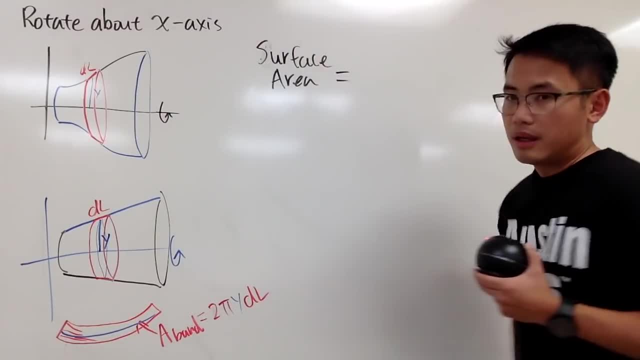 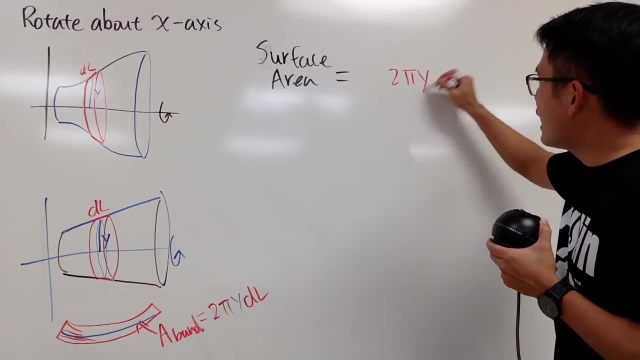 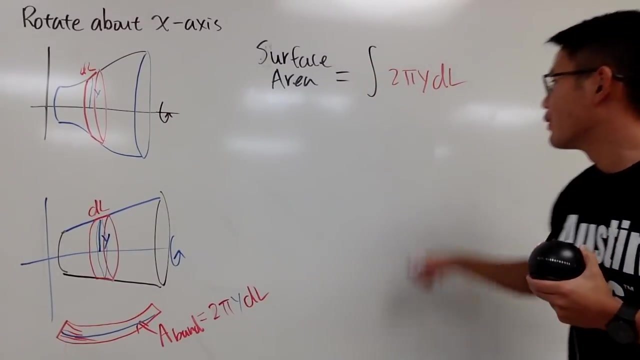 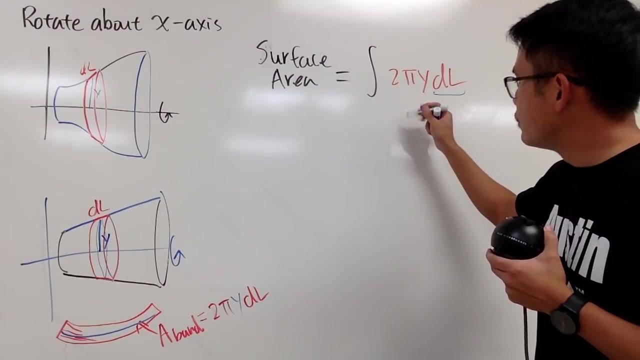 let's do the surface area now. Well, this is the area of the band, which is that You need to put that down, which is two pi Y times DL, And, as always, we have to integrate. But here's a trouble. we are in the l world and this is like the art length video: focus on the dl. we have two. 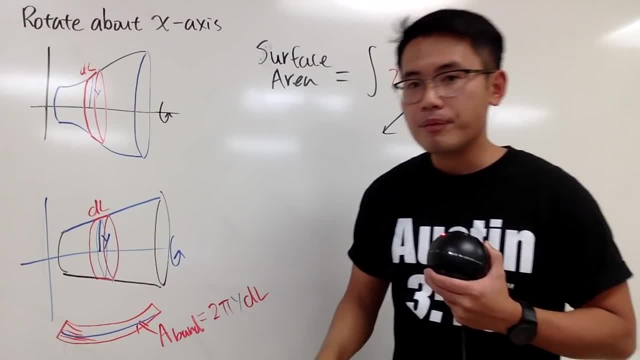 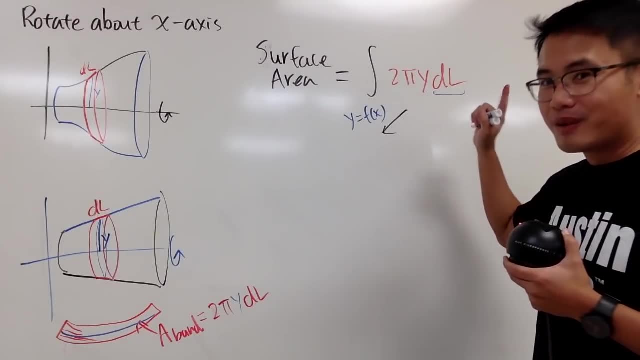 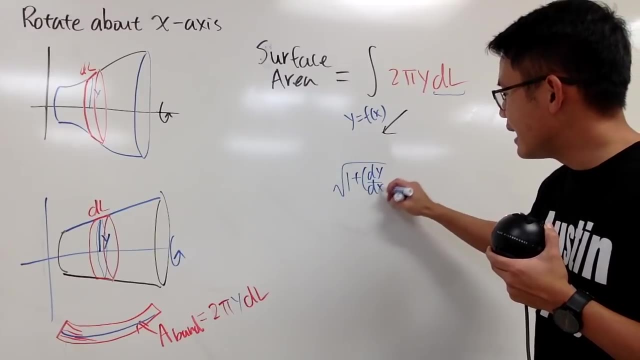 situations, because this curve right here could be described as y, as a function of x. remember, for the dl part, we are going to just open the square root and then we put on one plus dy, dx, and then you square that and then you have the dx right here and this will be for the dl when you 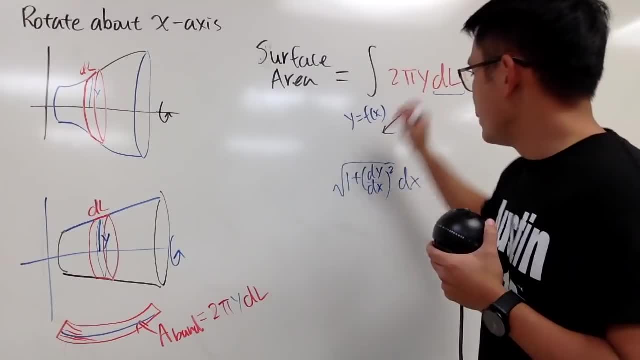 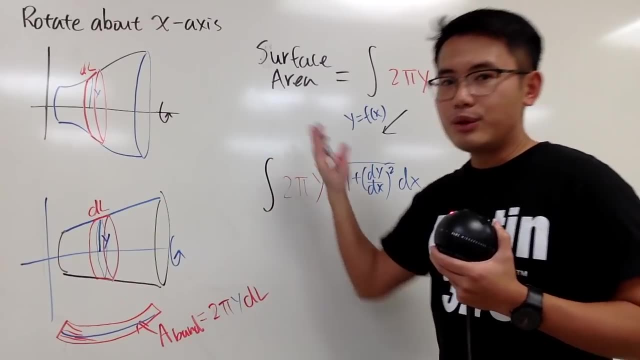 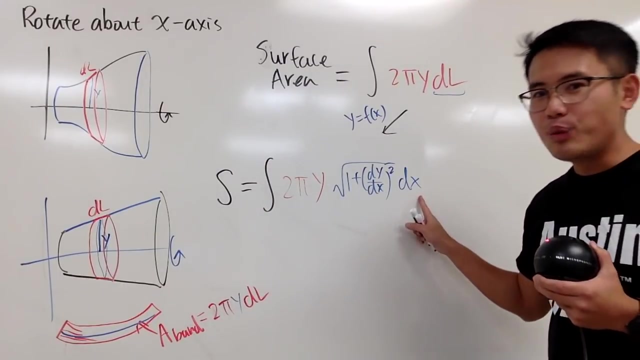 have this situation and then the rest pretty much stays the same. we have 2 pi y and then, of course, we have the integral, and the usual notation for surface area is capital s. that's my s, this is my integral. anyway, look at, we are in the x world. so i will have to come here and look for the x value.